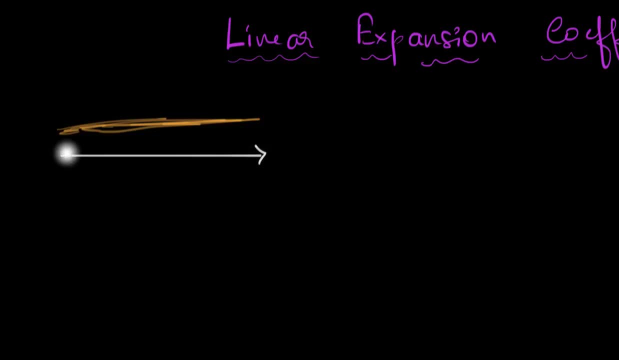 Say, it has a length L And it's sitting on your desk at some temperature T. Now you decide to heat this thing up. So you have a gold wire and you heat it up, And when it heats up its temperature rises. 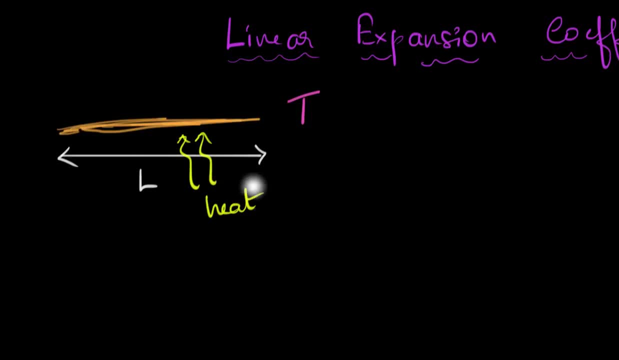 and the whole thing expands and you can see it expanding. So as you heat it up, we will see that the wire starts expanding like this. Okay, let's put that thing over here. This is the expansion, This is the expanded wire. 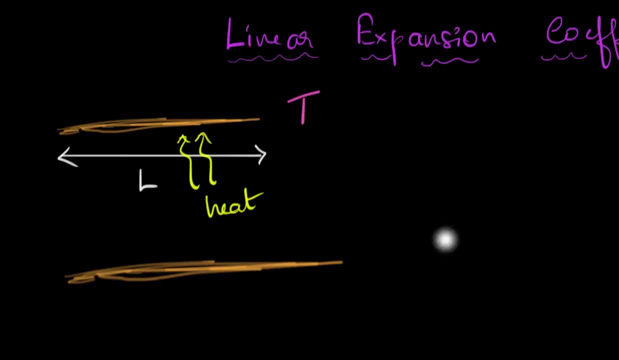 And since the temperature has increased, now the new temperature, let's say, is T plus delta T. Delta T represents the change in temperature, how much the temperature increased. And now we'll compare the length of this wire to the previous length. 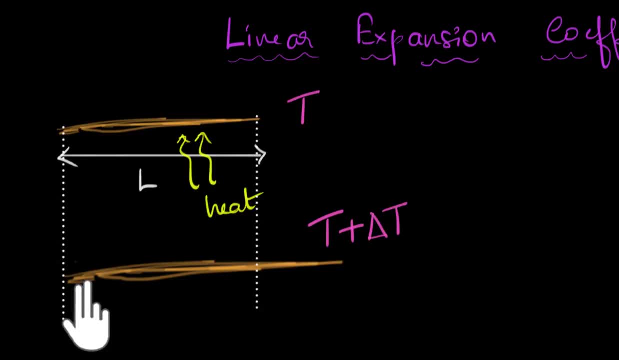 Now, this is how long the wire was initially, So this would be L And due to the expansion, this is the extra length, So let's write that down: This would be L, This is L And this, this region, is that extra length, delta L. 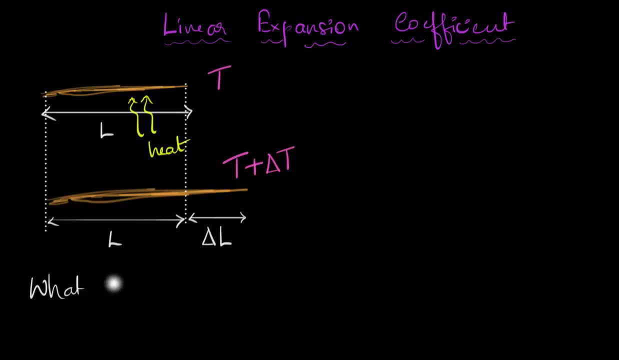 And the big question now is: what does delta L depend on? Let's think about this. We know that the wire expanded because we increased the temperature. So we could say that more you increase the temperature, more the wire will expand. In other words, we could say that more the value of delta T 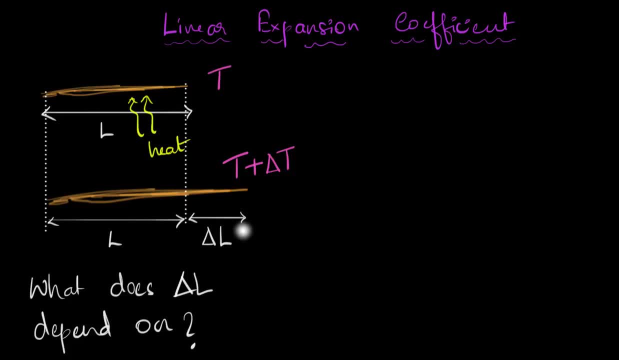 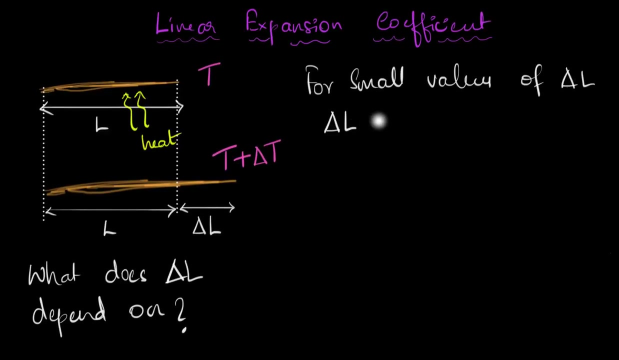 more the value of delta L. right Well, experiments support this. In fact, it turns out that for small values of delta L, for small values of delta L, it's even found that delta L is proportional to delta T. Proportional to delta T. 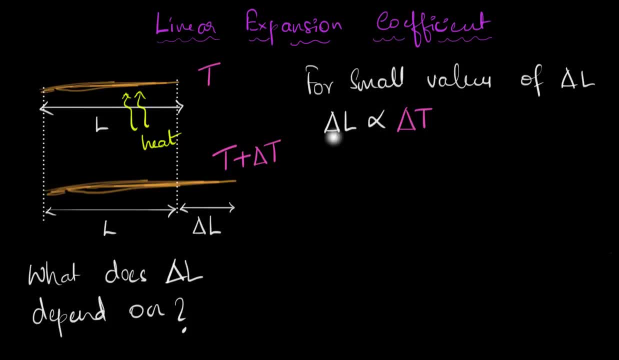 And what I mean by this is that if you double the value of delta T, then delta L will also double, And you may be wondering: well, what does that mean? What do you mean by small values of delta L? How small is small? 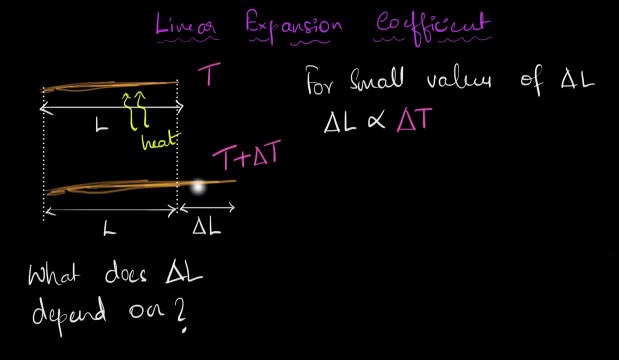 Well, as long as the expansion is much smaller than the original length, In other words. in other words, as long as delta L is much smaller than L, this will hold true, Not like what I've shown in this diagram Over here. delta L is considerably large. 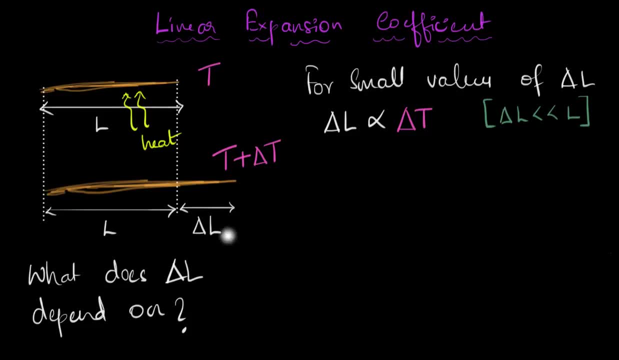 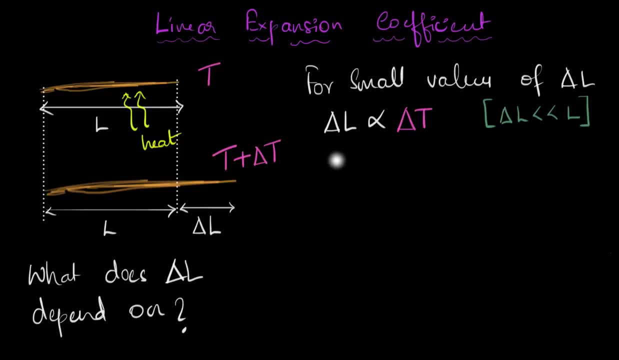 But we will see. in reality, delta L is very tiny compared to L itself. Okay, All right. anything else that delta L depends on, Hmm, turns out. there's one more thing delta L will depend on. Delta L turns out to be also proportional. 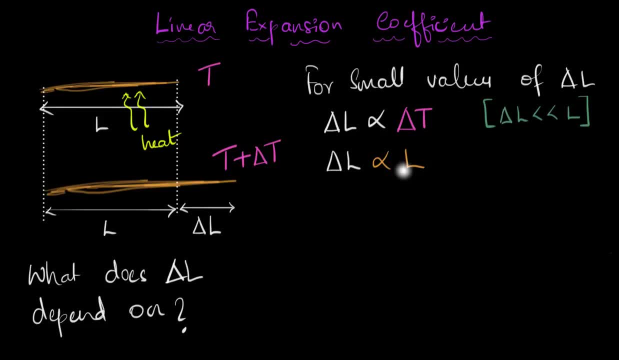 to the original length, And you may be like whoa, wait a second. Why would delta L depend on L? Well, if you think about this, it'll make sense. Imagine that we started out with a wire of not length L but length 2L. 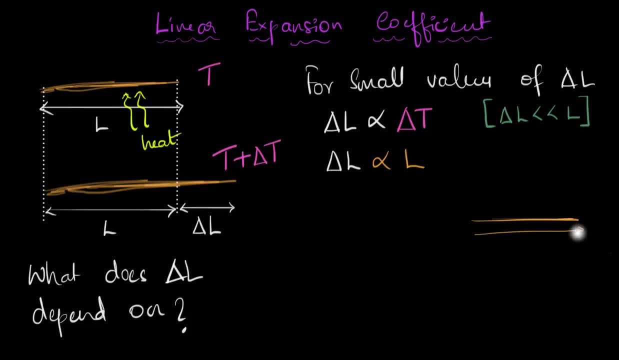 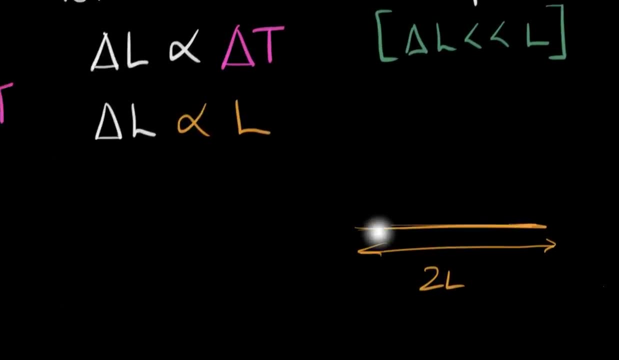 Think about this. Imagine we had a wire gold of length 2L. And imagine again: we heated it up and increased temperature by delta T. We could assume that this wire is made up of two wires, each of length L, right? 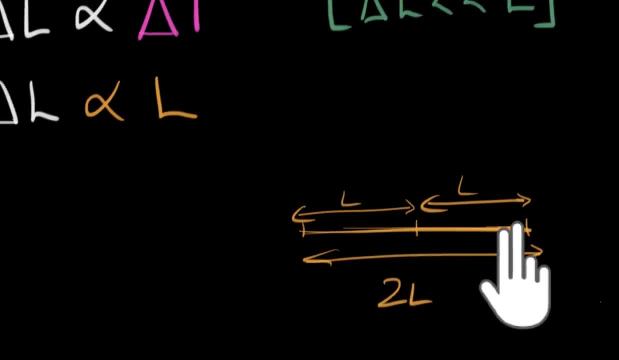 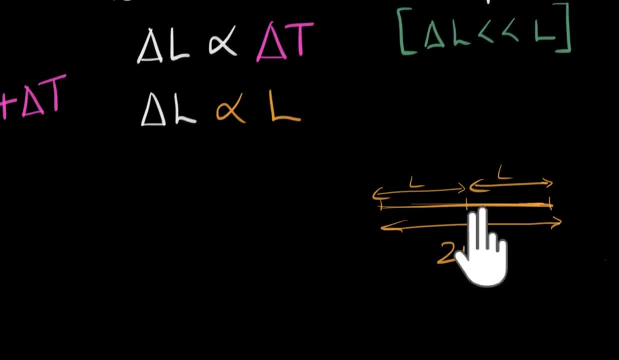 We could do that, And since we know that each wire, or each section of the wire, is going to expand by delta L, we will see that this section will expand by delta L and this one will expand by delta L as well. 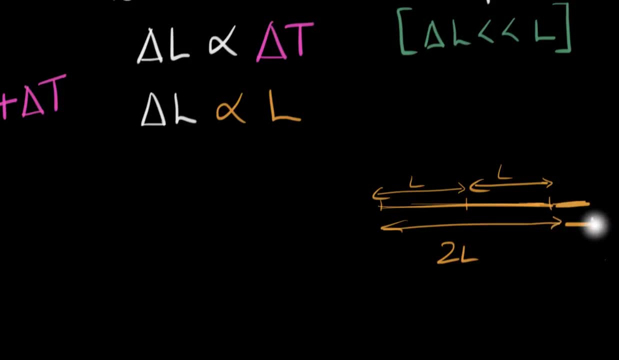 Therefore the total expansion- do you agree- would be 2L. So if you double the length of the wire, the expansion doubles, And if you triple it, this would triple. So in other words, delta L, or the expansion in length. 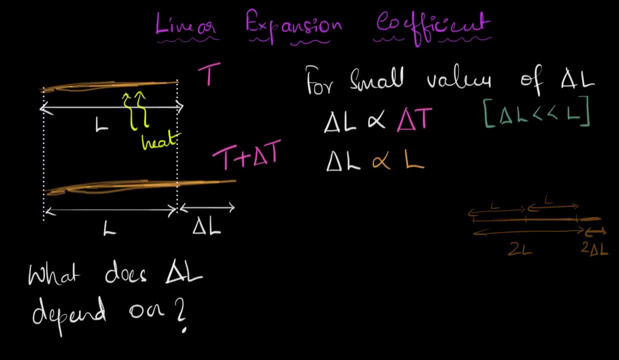 is proportional to the original length of the wire. So if we put these two together we could now say delta L is proportional to L times delta T, And we could now replace this proportionality with an equal to sign by putting a constant over here. 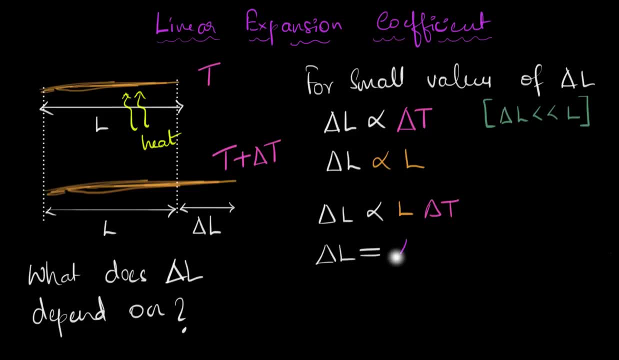 And that constant can be used. any letter can be used for that. Over here we're going to use alpha L as the symbol for the constant times L, delta, T, And this expression now is going to help us calculate how much something expands on heating. 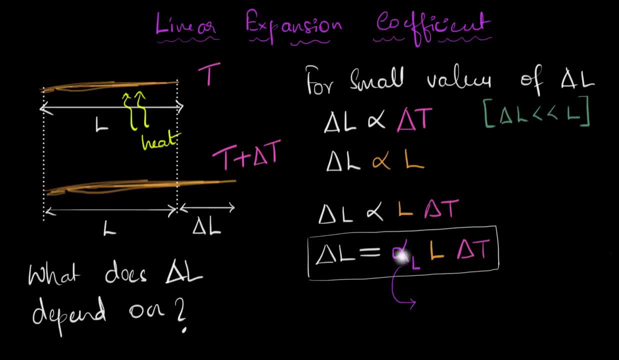 And this constant alpha L is what we call as the linear expansion coefficient. So let me just put a short form over here, I won't write it again. So, linear expansion coefficient. This is linear expansion coefficient. All right, now let's get to know alpha L. 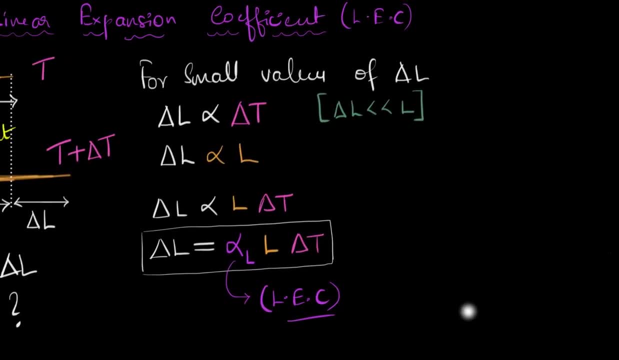 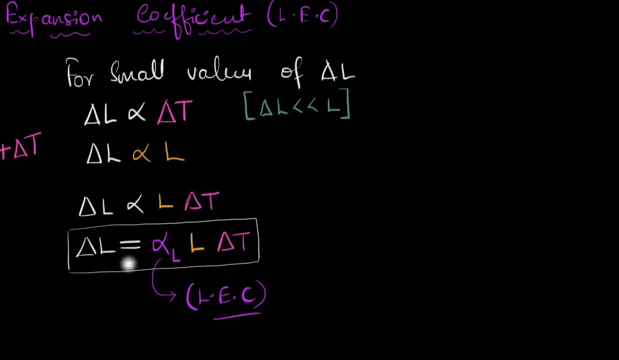 a little bit better. So let's put this thing a little bit aside. Okay, The first thing we'll do is figure out the units of alpha L. We can do that by dividing both sides by L delta T, So we'll isolate alpha L. 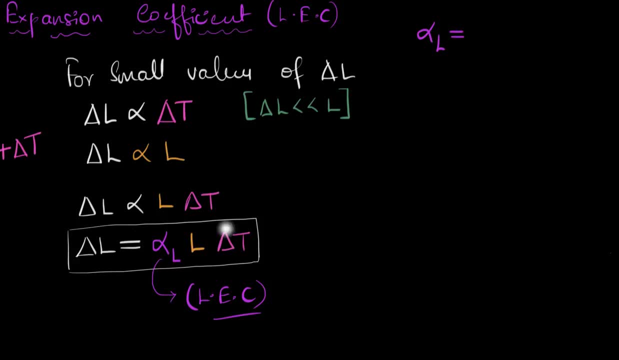 So if you divide both sides by L delta T, the right hand side it would be alpha L, which I'm writing over here, And the left hand side would be delta L divided by L delta T. Divided by L delta T. 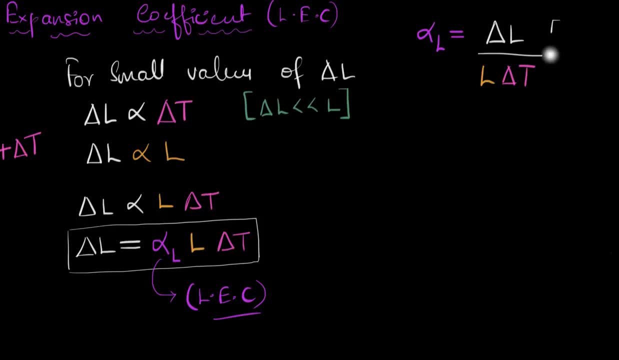 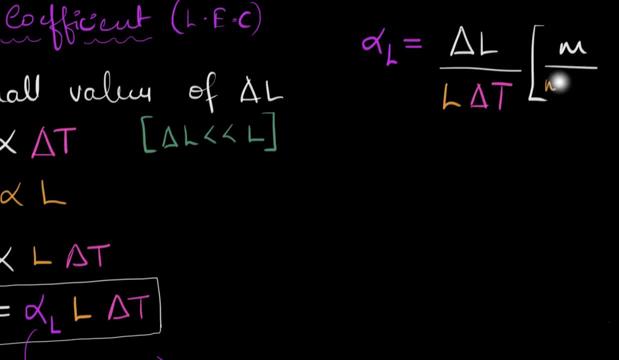 And from this we can now figure out the units of this. Let's see: Delta L has the units of well, its length, So it's meters. L is also length, That's also meters. And delta T temperature. 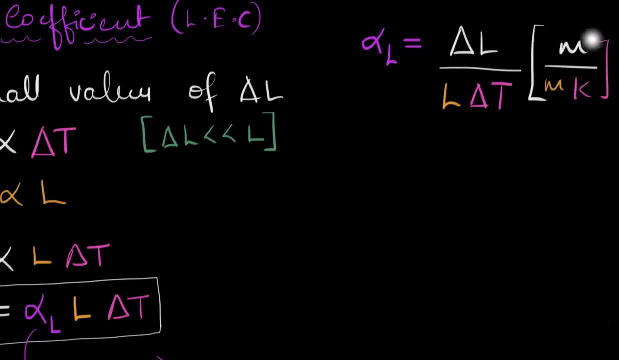 well, the standard unit is Kelvin, So this cancels, which means we end up with one over Kelvin Or Kelvin inverse. That's the unit of alpha L, the linear expansion coefficient, For example. for example for gold, for gold. 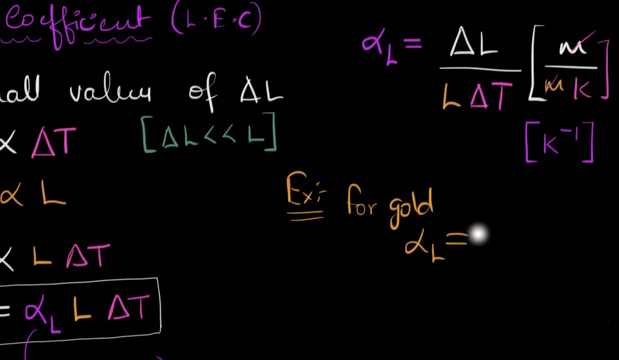 it turns out that alpha L values- I just looked it up- is equal to approximately 14 times 10 to the minus six Minus six Kelvin inverse, And this might seem a little bit weird as to what do we even mean by 14 times 10 to the minus six? 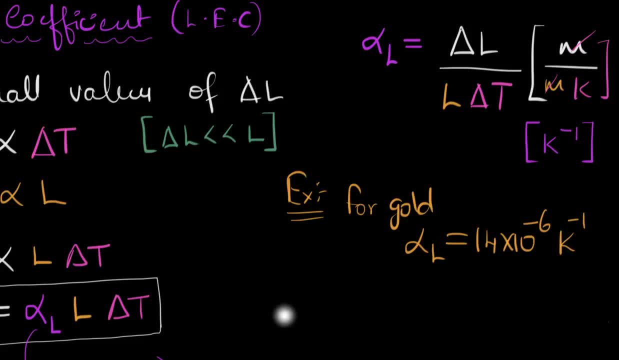 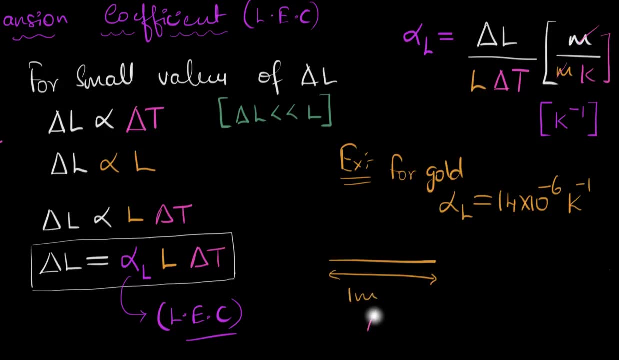 Kelvin inverse. Well, what it means is if you took one meter long wire, one meter long gold wire, and if you increase this temperature by one Kelvin, then notice: L becomes one, delta T becomes one, which means delta L becomes equal to alpha L. 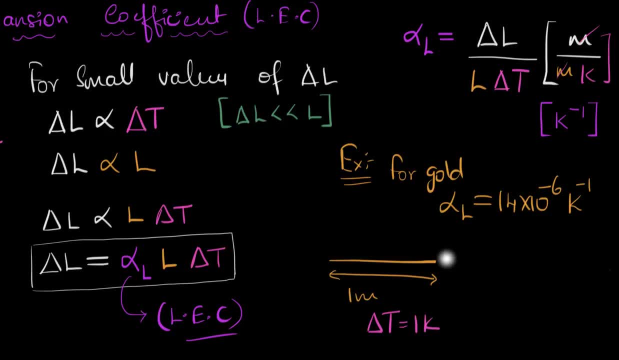 And therefore, in our case, the expansion in the gold wire, this expansion extra length, the expansion in the length would be this number 14 times 10, to the power minus six meters. This is meters, because this is meters. 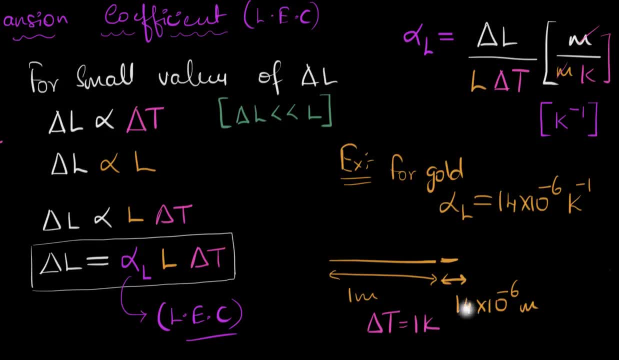 So the alpha L, the linear expansion coefficient, tells us how much a one meter long wire, when increased the temperature by one Kelvin, would expand. That's what this number really is, And it doesn't have to be meters. This could have been one feet. 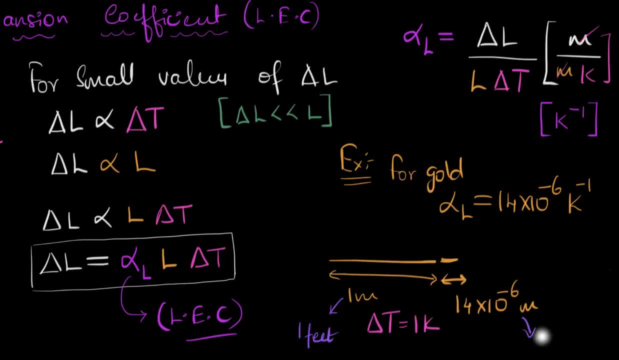 If this was one feet, then this would be 14 times 10 to the power minus six feet. So whatever unit of length you take, same unit of delta L you end up with. So more the value of alpha L, more the material expands on heating. 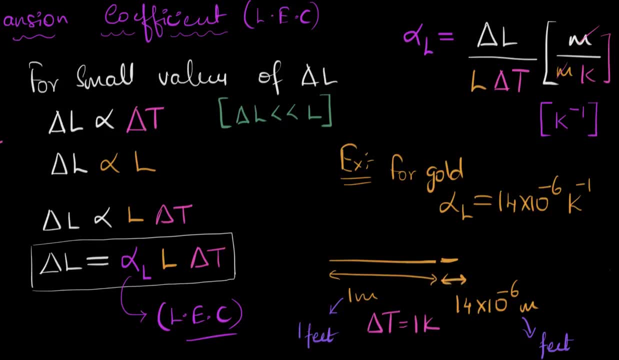 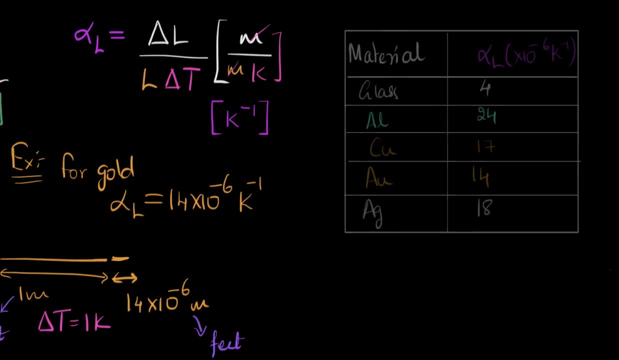 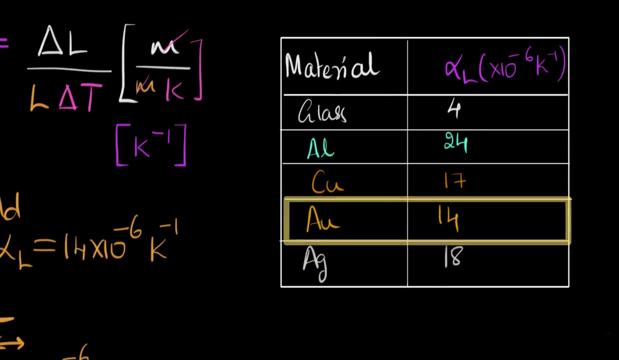 or more sensitive the material is to changes in temperature. So now let's look at some values of alpha L of some typical materials. So here it is. We have alpha L values in terms of 10 to the power minus six Kelvin inverse, 14 times 10 to the power minus six Kelvin inverse. 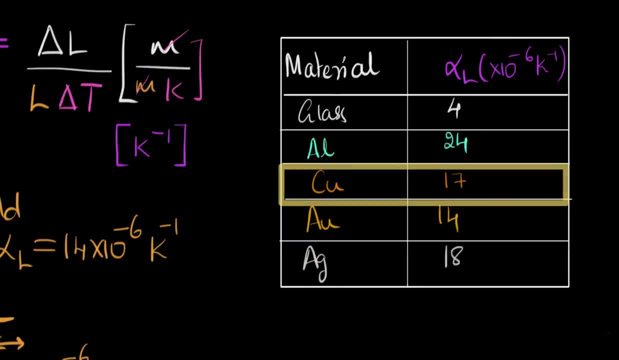 Look at copper: It's 17,, which means copper expands more on heating compared to gold. Aluminium expands even more. And look at glass: Its value is just four times 10 to the minus six Kelvin inverse, which means glass doesn't expand as much as these metals do. 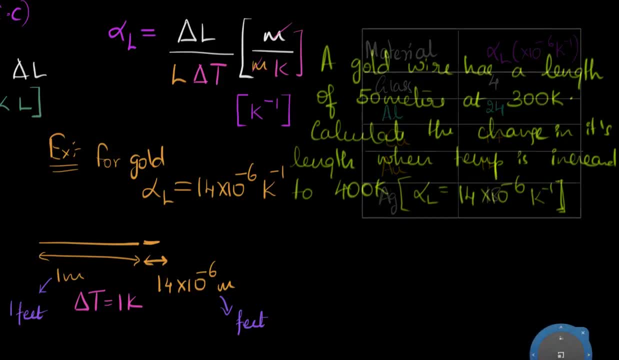 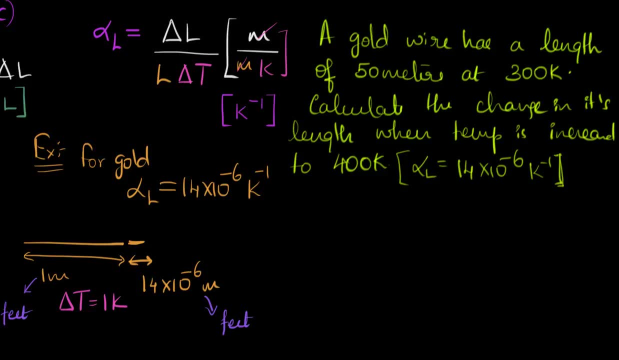 All right, I want to end this video with a simple numerical. Here it is. So we have a gold wire which has a length of 50 meters at 300 Kelvin. We have to calculate the change in its length when the temperature is increased to 400 Kelvin. 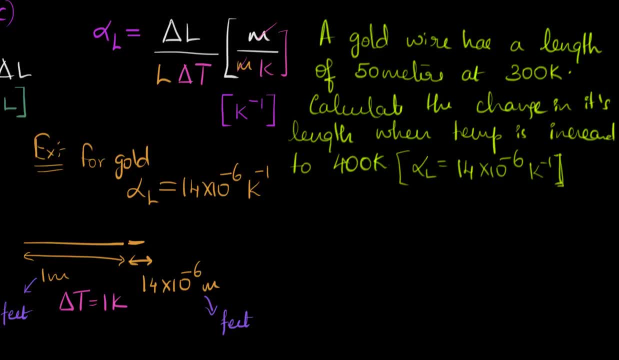 Alpha L value is given. It's the same thing, It's gold. I want you to pause this video and first see if you can try to figure this out yourself. Try to do it intuitively. All right Time for solution. We know that alpha L 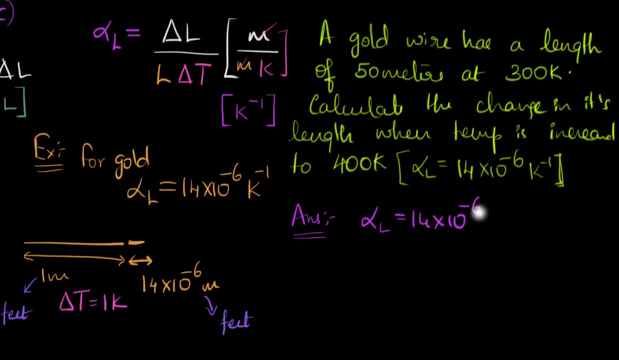 it's given to us is 14 times 10 to the minus six Kelvin inverse, which means if we have one meter long gold wire and increase the temperature by one one Kelvin, then the expansion would be 14 times 10 to the minus six. 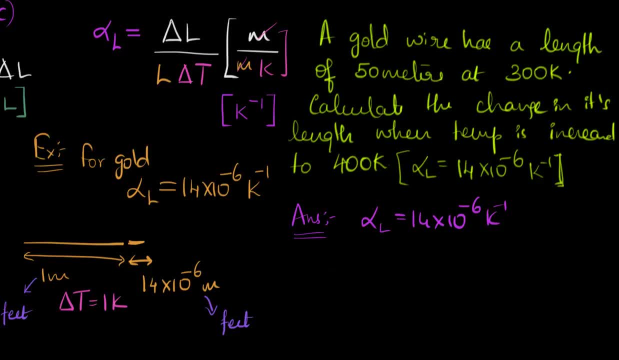 meters, But we have 50 meter long wire. Ooh, that means now, if we had increased the temperature by one Kelvin, the delta would be 50 times this number. Does that make sense? For one meter it would be so much. 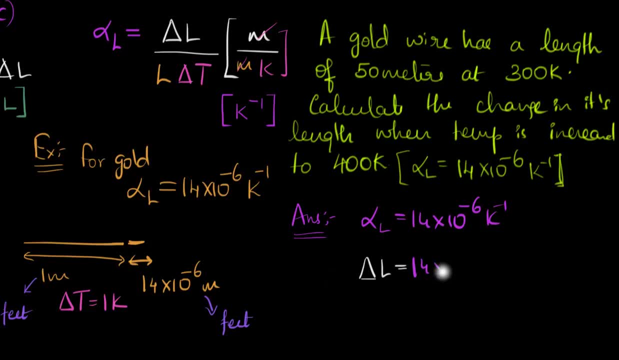 For 50 meters it'd be 50 times that much. So it would be 14 times 10 to the minus six Kelvin inverse multiplied by 50, 50 meters. But this would be the expansion in the length of the wire. 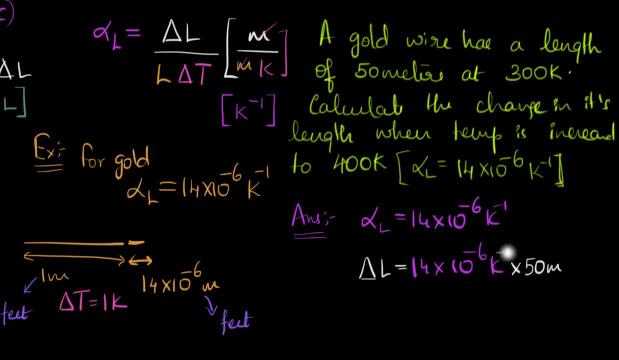 So this would be the expansion in the length of the wire. This would be the expansion in the length of the wire. So we now know the length for one Kelvin rise. Right, For one Kelvin. Per Kelvin means one Kelvin rise. But how much Kelvin rise do we have?